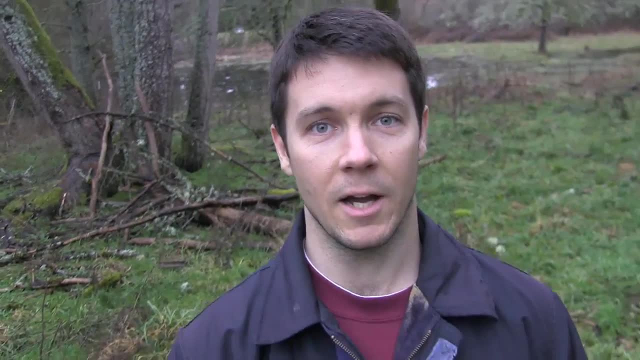 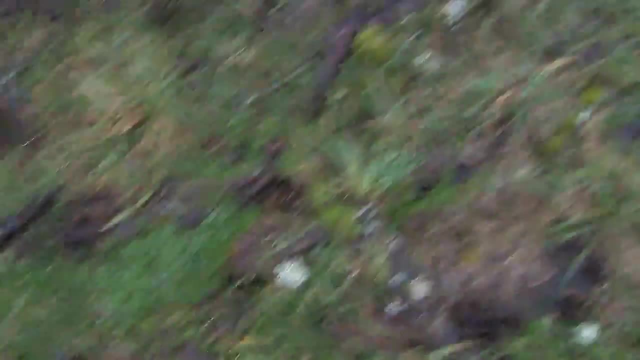 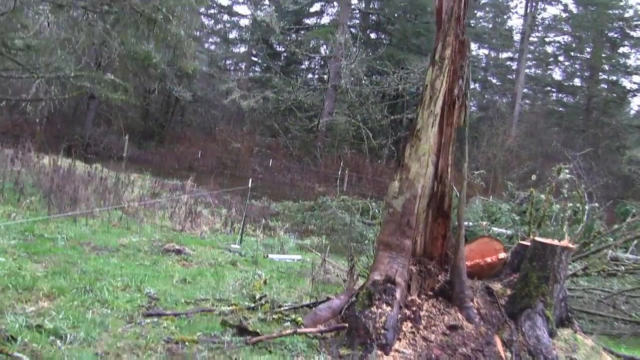 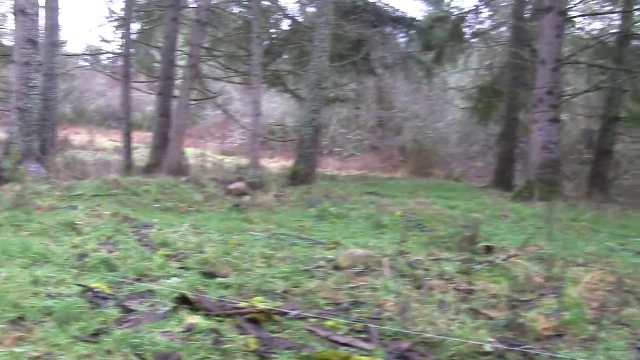 If you look behind me here, you can see that- I think you can see it in this camera. here there's some water and it's kind of I don't know. it's probably a foot deep over there, And then if you look around over here, we've got some water right down in that area too, along the fence line. Now I would like to direct all that water around this big raised up area of land all the way down to that area right now. But my concern is is this: 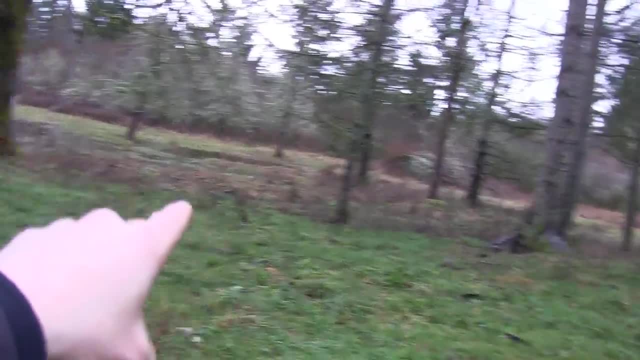 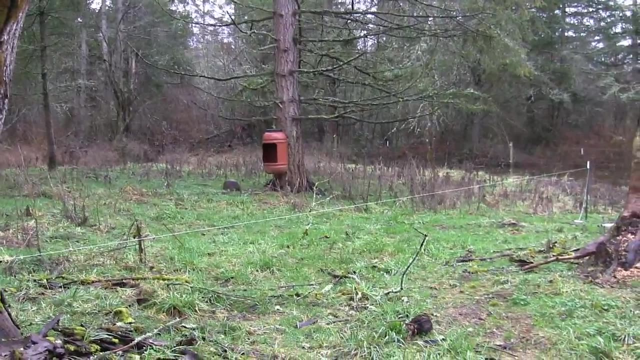 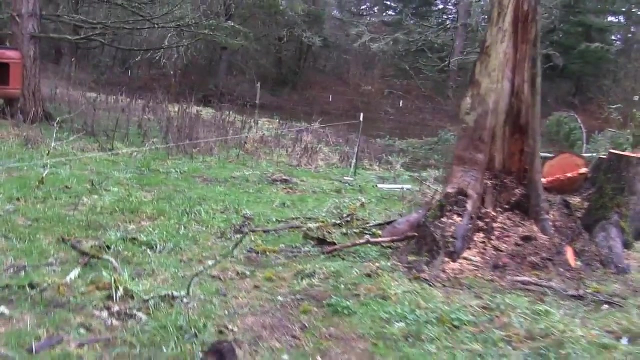 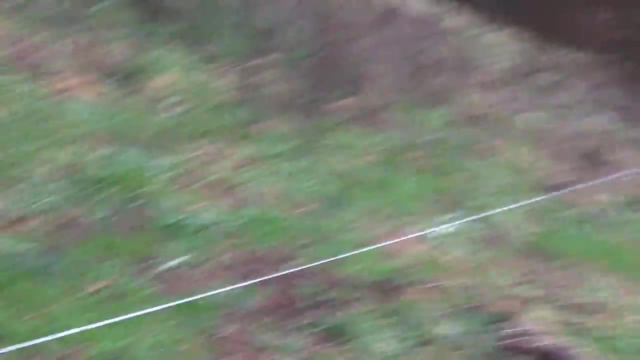 area right over here that I'm pointing out, lower than the area over here. So we've got to figure that out And, like I said, I don't have any expensive equipment, So we're going to do this the old fashioned way. Now I already went and got some T-posts- you can see right there- and pounded it into the ground And you can see the line on there. I run it all the way down And it's attached to another T-post down at the 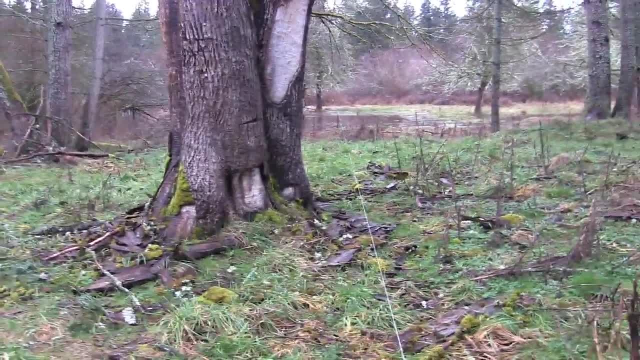 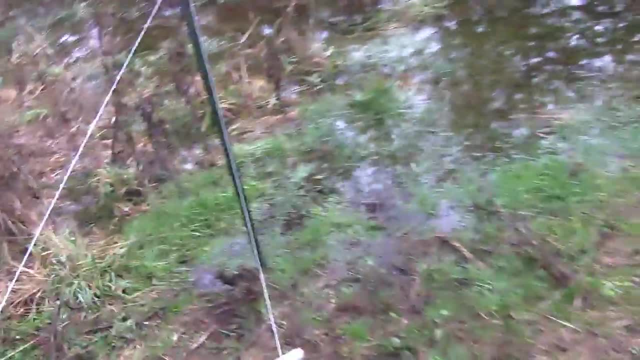 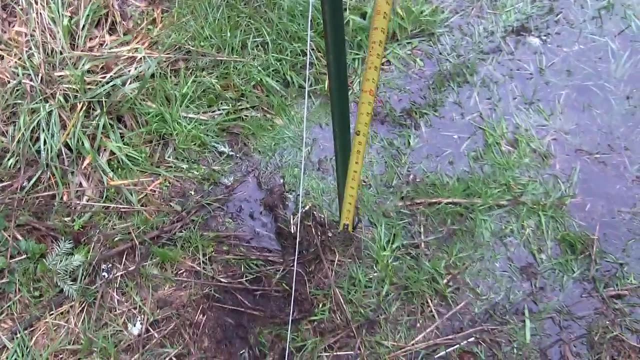 the other end there. so what we do is put those two t-posts in the ground and then measure with a tape measure from the bottom of the t-post. see if we can figure this out with one hand. all right, so i'm gonna go down at the base of the t-post and i've got both t-posts pounded in, right? 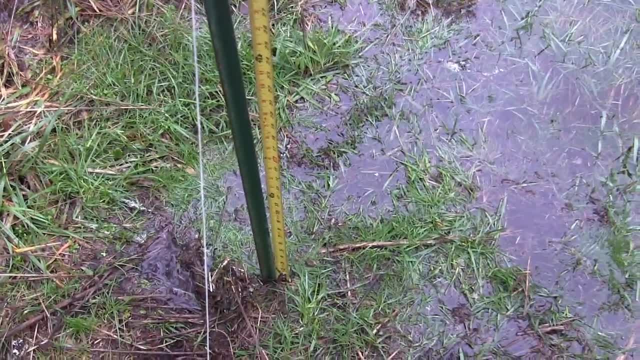 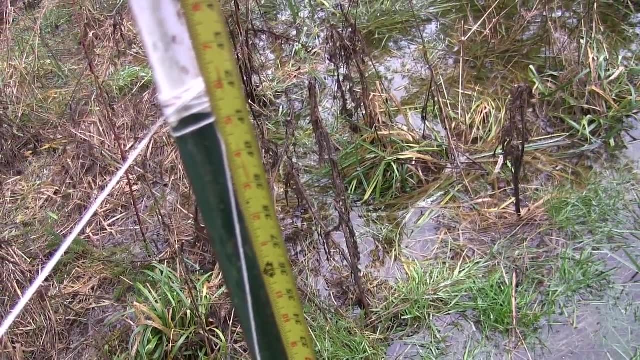 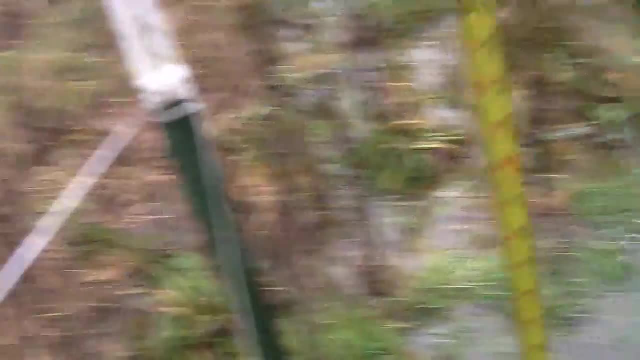 at the edge of the top of the water there. so i'm going to measure up. and i measured up on both of them to it's just an arbitrary number- 41 inches, and that's where i have my line attached, right at the 41 inch height. then i went and did the same thing down there. i put a t-post in. 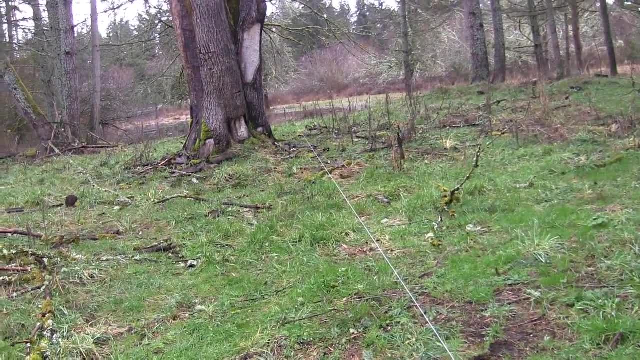 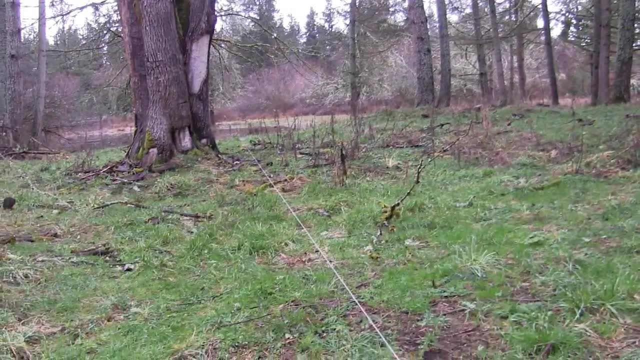 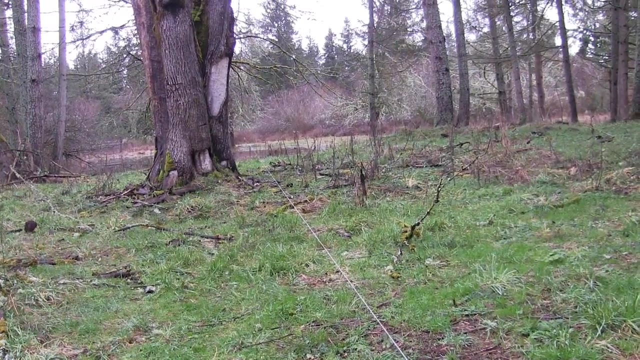 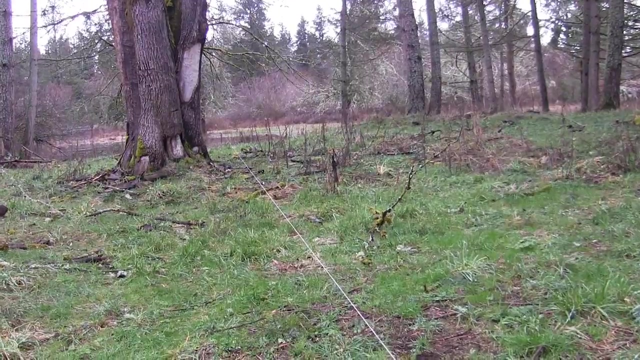 and measured 41 inches up from the water line and attached the line to that end. i pulled this line super tight. i mean it is really tight, but because there's obviously a you know a little bit of weight to that line, i think no matter how tight you pull it, you're gonna get just a touch of bowing to it. i mean it's pretty. 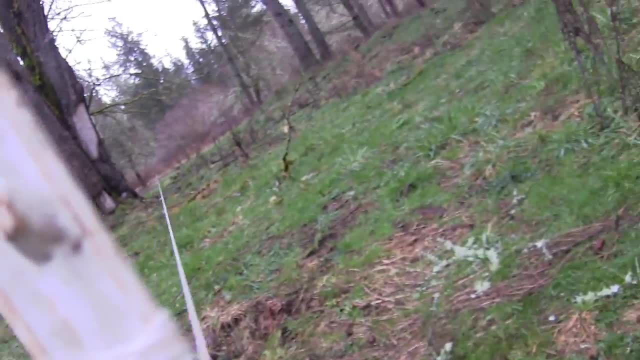 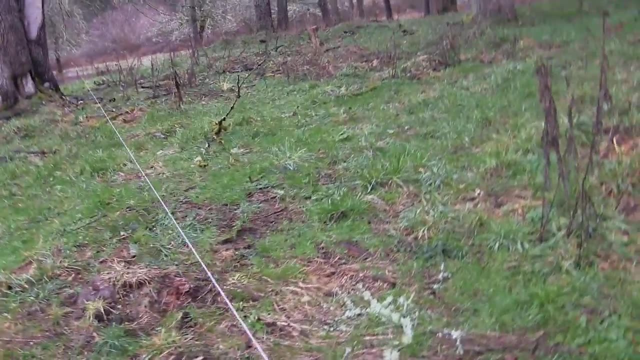 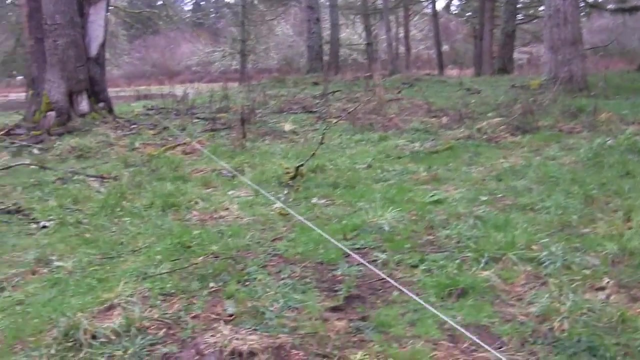 straight. you may not even be able to pick it out- i can hardly with my naked eye- and maybe, yeah, i mean it's pretty straight, but there's always going to be a hair of a sag in it just because there is weight to it. so what we'll do next is run out there to the middle of the line. 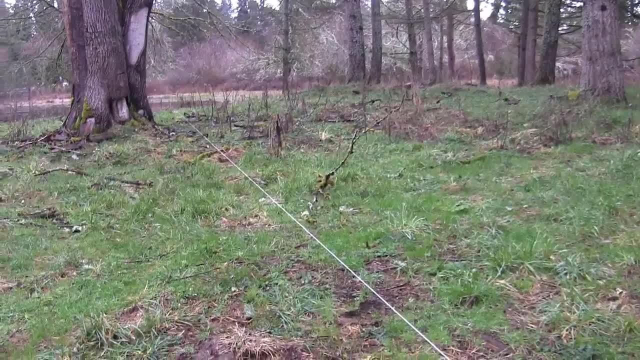 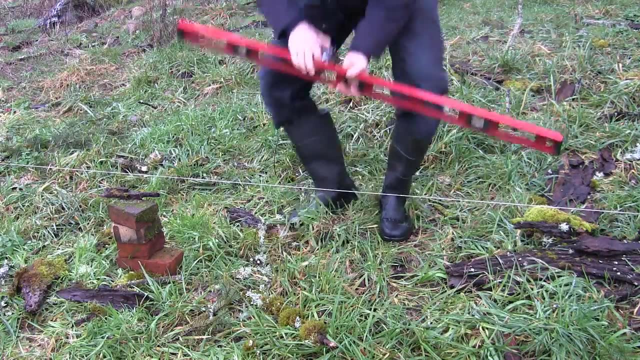 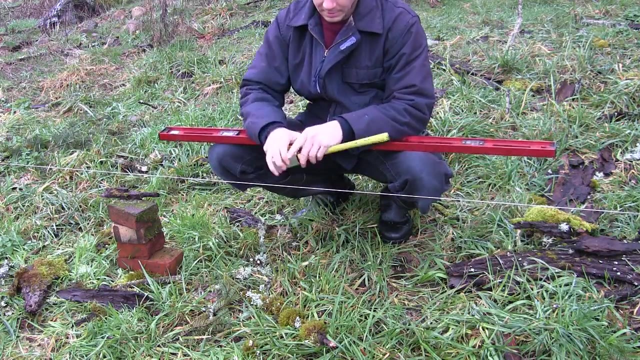 to make it as accurate as possible and grab our level and see where we're at, all right guys. so this is pretty makeshift, but you can get pretty accurate on this. so i'm going to get the tape measure out here and we're about in the middle of that line here. 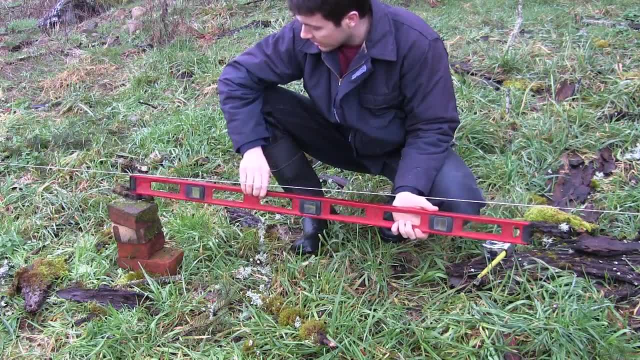 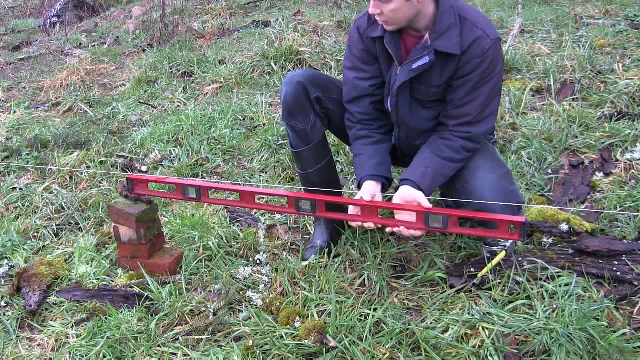 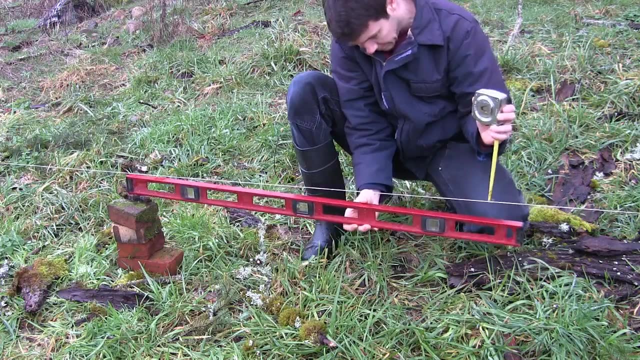 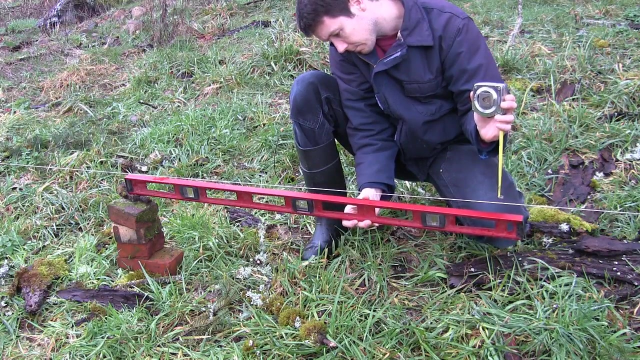 i've set up some bricks and a little piece of bark here to try and kind of balance that level just underneath the line and then i want to bring this thing up just to as perfectly level as i can get it and then measure the distance on this end over here. 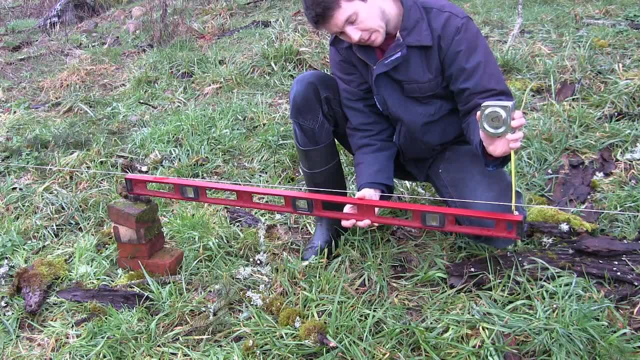 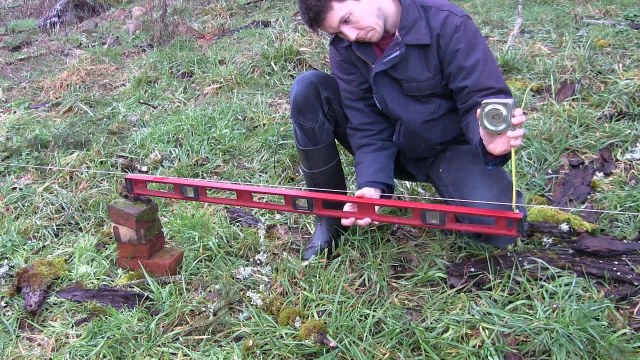 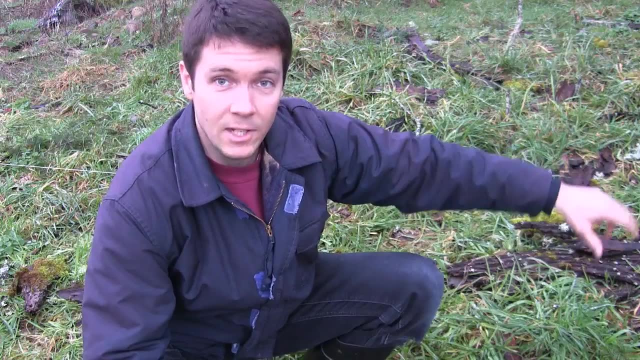 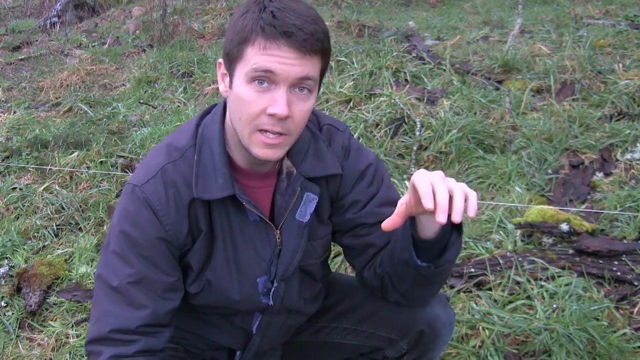 between the string and the top of the level, and i'm getting right at an inch. so now that i've measured that distance, i've got an inch gap between the top of the level and the string. uh, on this end over here, and so i know that for every 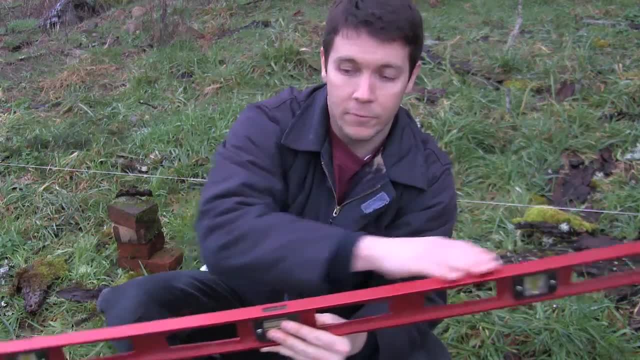 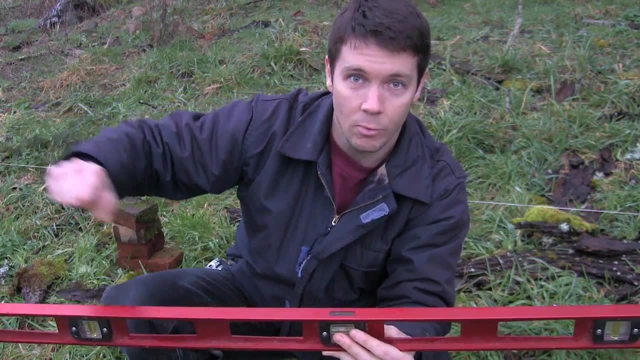 four foot. this level is four foot long, so i know that for every four foot of distance i drop one inch, going the way i want it to, to where i want to direct the water. so All you would do from there- and I already measured this out- 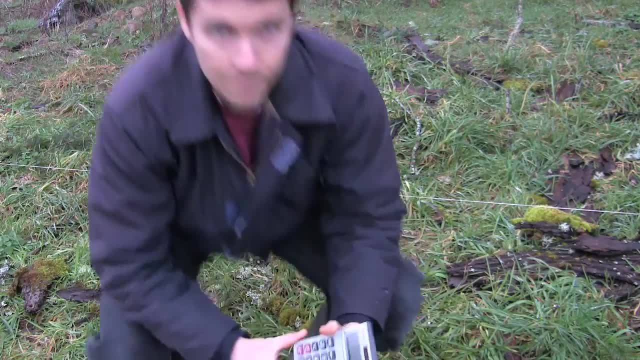 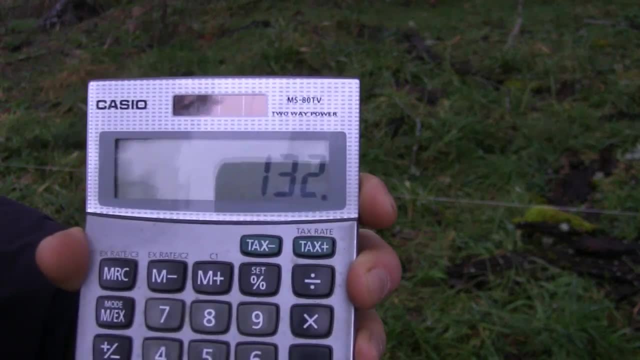 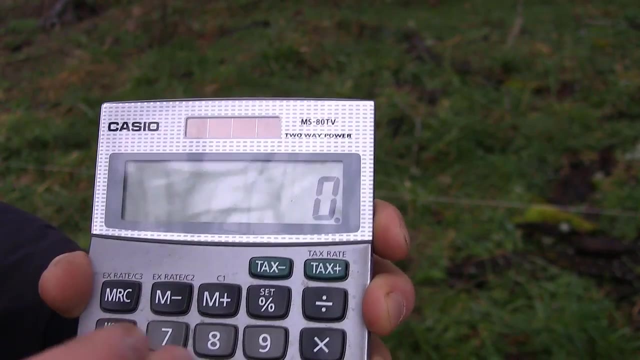 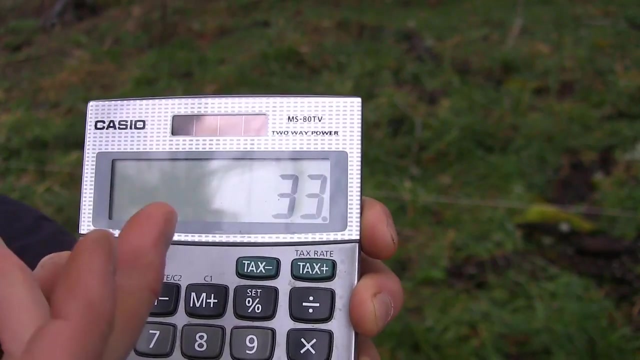 Get out of calculator here. so I've got, let's see, 132 feet From one end of the, from one stake to the other out there. so then all we do is just divide that by 4. look, 132 divided by 4 We get 33 feet, and so I know that for every. 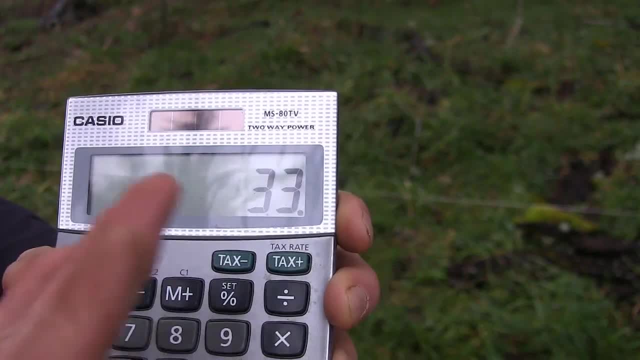 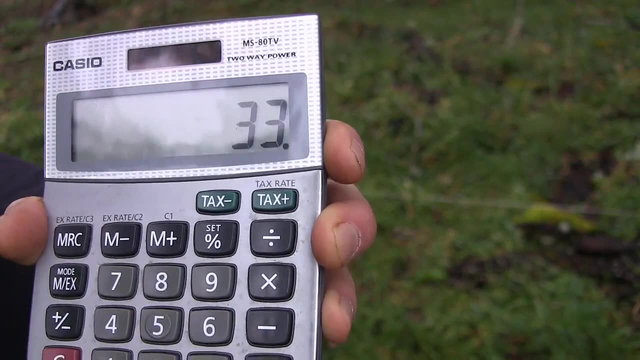 4 foot. I've got 1 inch and drop. so if I divide it by 4 I get 33. I've got 33 inches of drop overall from the top of the water down on one end of the top of the water on the other end. divide that by 12.